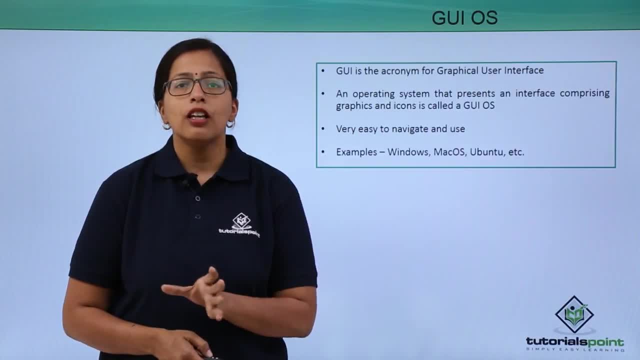 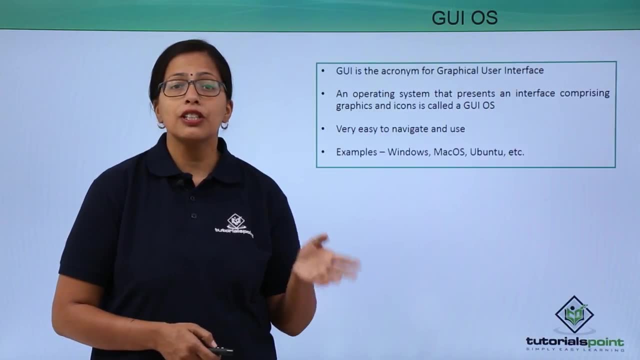 was developed by the command line interface, the MS-DOS, But the users found it very difficult to use. So Microsoft came up with Windows, the first GUI or the graphical user interface operating system. What was different here? The users did not have the ability to use the GUI OS. 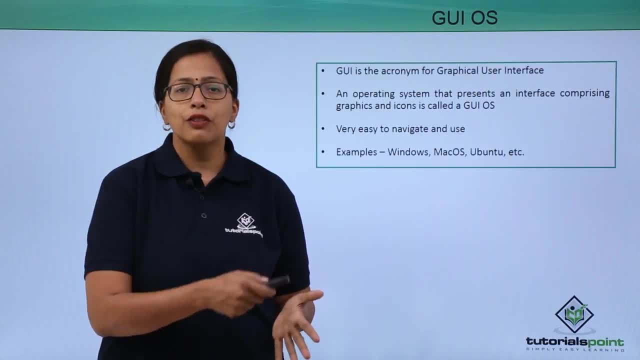 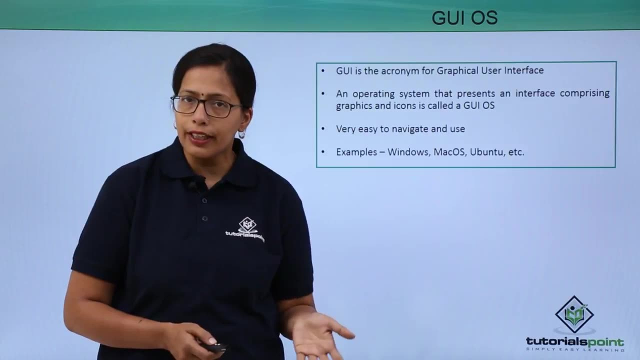 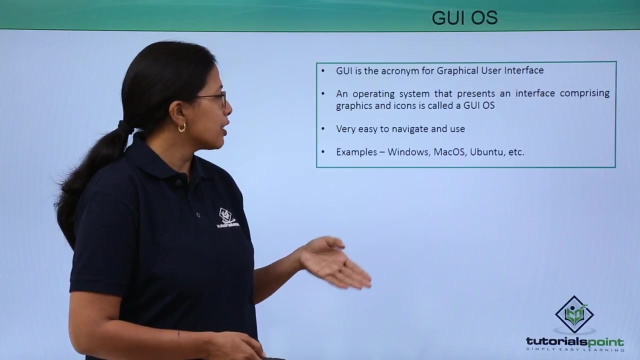 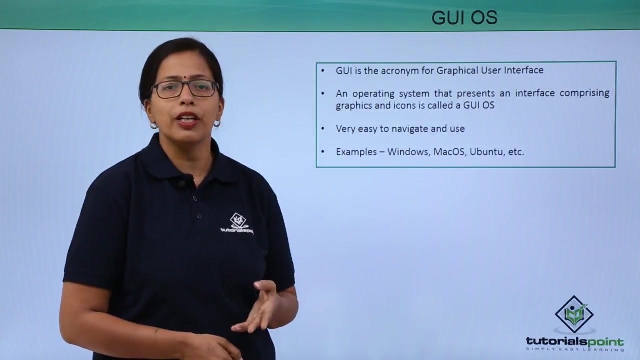 They had to remember commands to use the different parts of the operating system or open different software. Here just small small icons were given which could easily be clicked and those software or those things will just open up. So this was the GUI operating system Examples. as I told you, Windows, Mac OS, even Linux Ubuntu version is a GUI operating system. 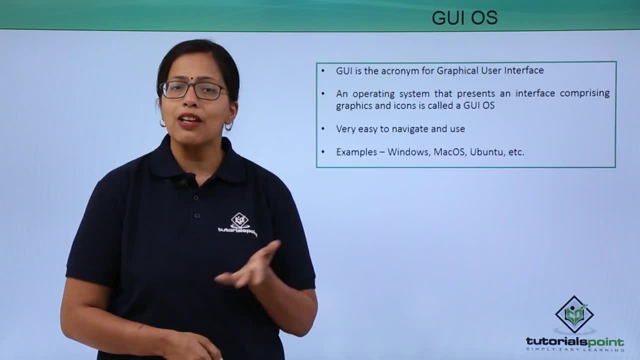 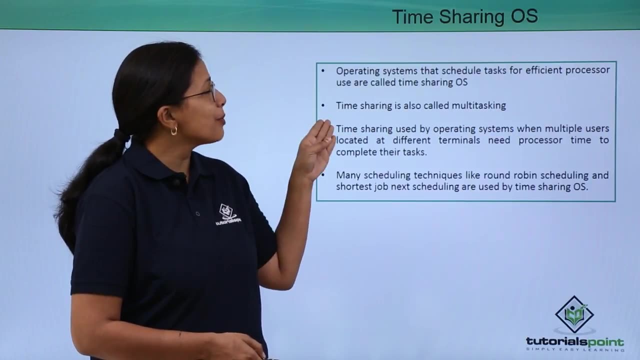 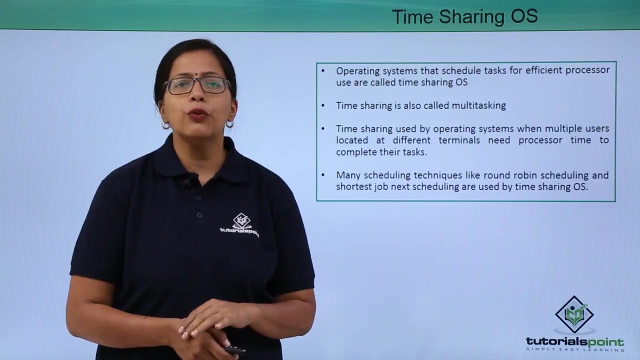 These have become very popular because they are very easy to use as well as navigate. Then comes the time sharing OS. What is so specific about it? Operating systems that schedule tasks for efficient processor use are called time sharing OS. In the previous video we 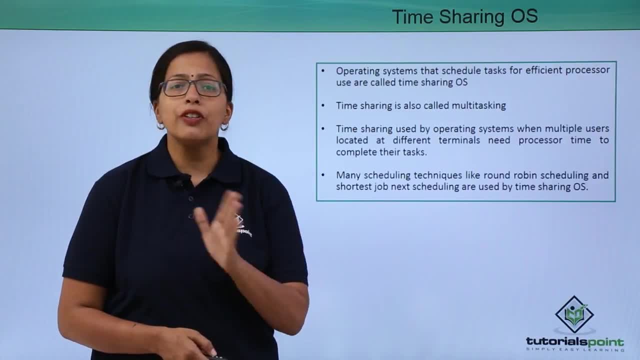 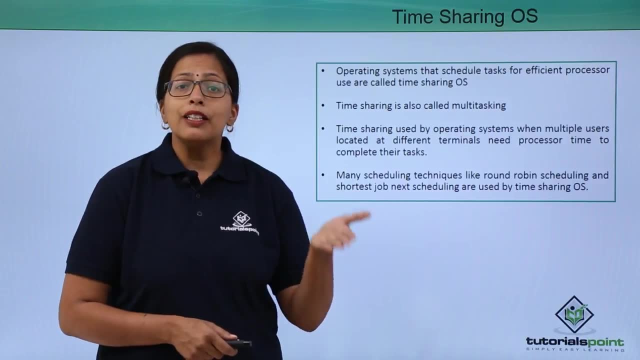 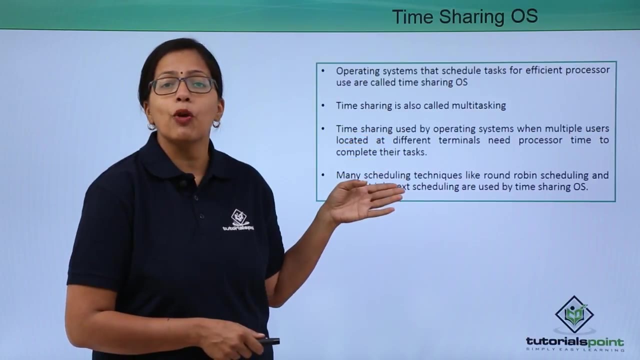 have discussed how the operating system manages memory time. What it does is it processes multiple tasks at the same time, So multiple tasks are sharing the same time slice in the processor. For this, a specific type of operating system which is called the time sharing operating system. 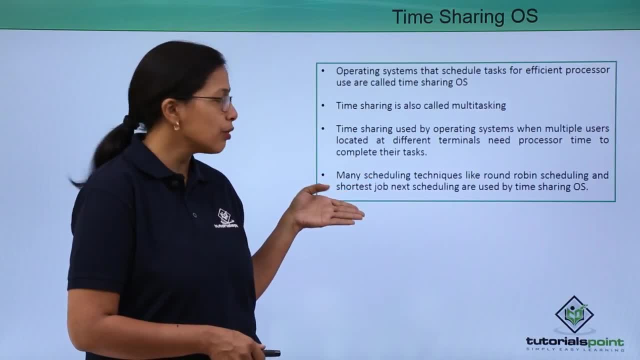 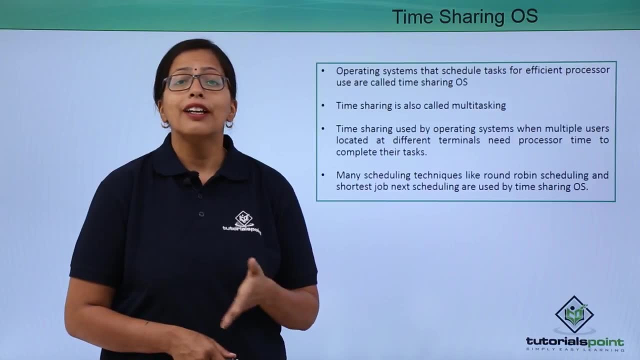 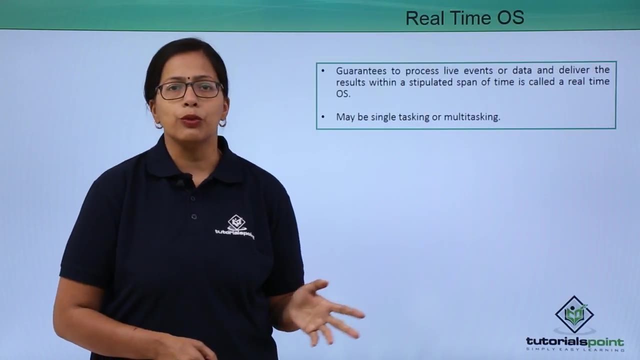 is required Here, as we have discussed in our previous videos many scheduling techniques like round robin scheduling or shortest job next scheduling or deadline next. These are the techniques that are used by time sharing operating system. Then we come to the real time OS, Real time. 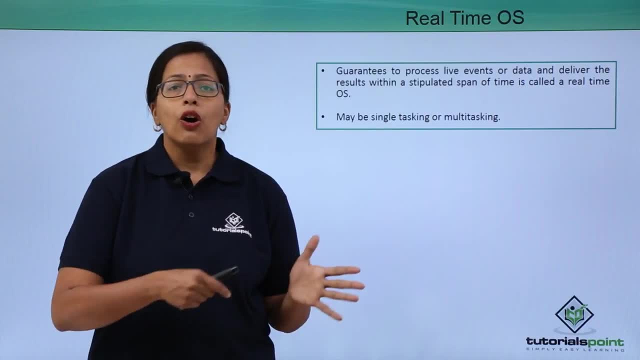 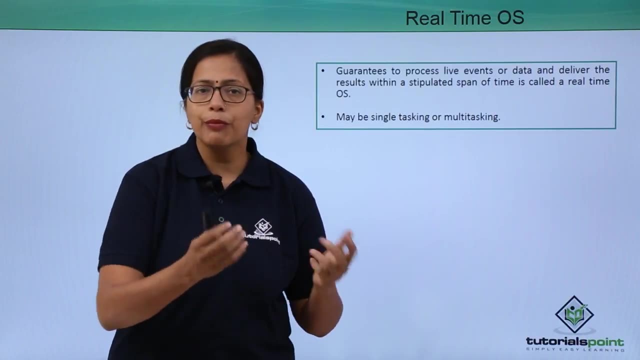 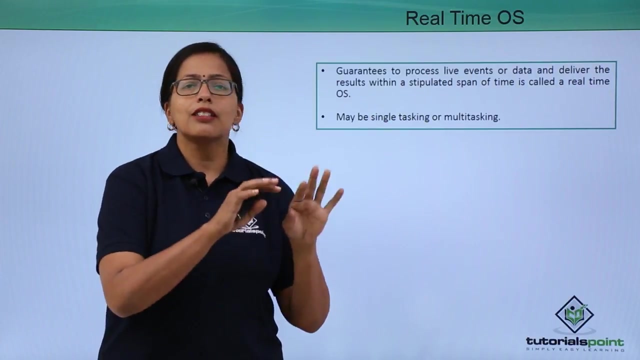 operating system. You know that many functions or many things are being done in the real life world today which need real time operation, For example, weather forecast. If you have a smartphone or even on your computer, you just go to google and just type the name of your place and 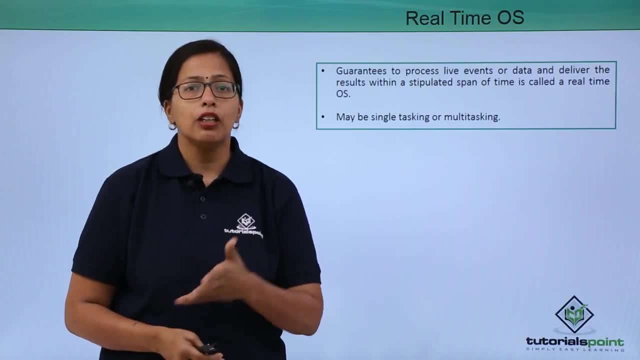 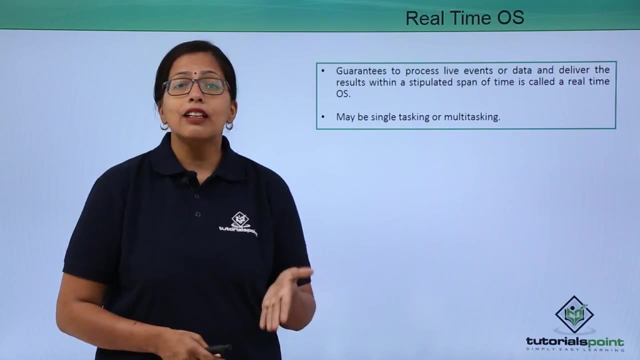 its weather, then immediately all the weather details will come. Now, somebody with who is sitting at a different place will get information about his or her own data. So that is a real time operation. The weather forecast that is currently now being done, which will be: different from one hour later. For that a different type of operating system, which is called the real time operating system, is used. Real time operating system could be single tasking or multitasking. That means it will take only one task or one job at a time, or it can take multiple.